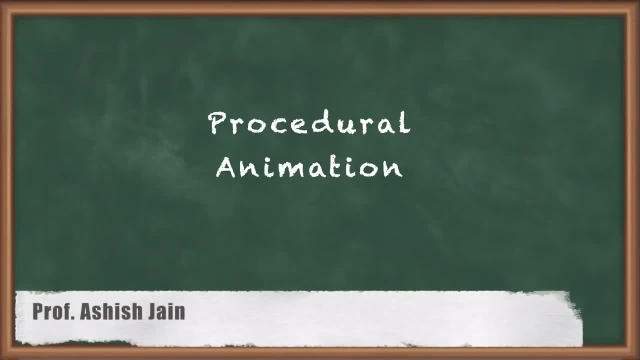 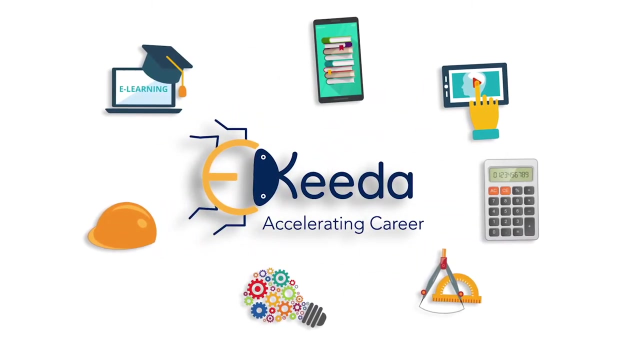 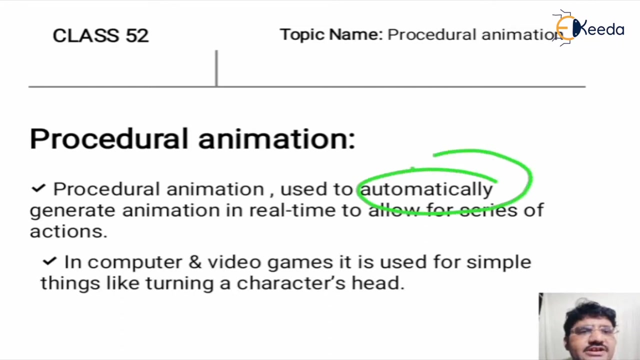 Hello friends, in the previous video we have discussed about motion control in animation- How to control motion in animation. Now, in this video, we are going to learn about procedural animation. So let's start. Procedural animation is used to automatically generate animation in real time. 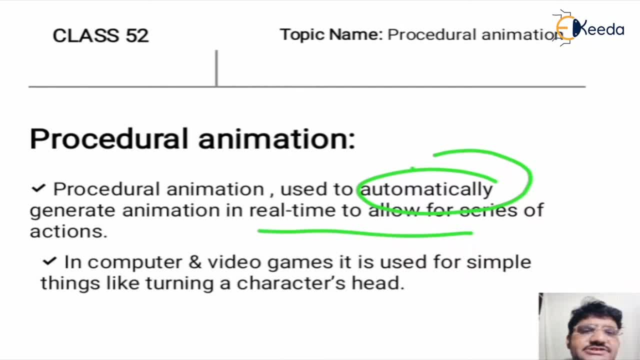 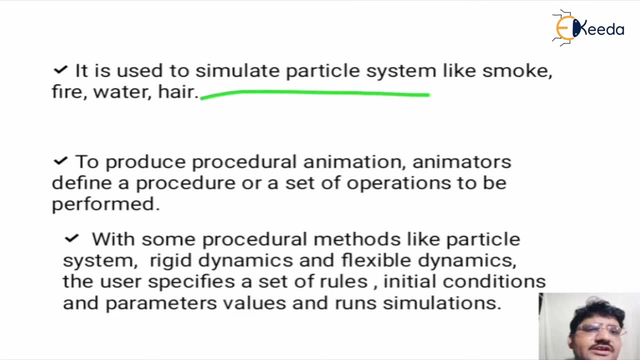 to allow for series of actions In computer and video games. it is mostly used for simple things like turning a character head. This method is used to simulate particle systems like smoke, fire, water, hair, etc. To produce procedural animation, the animators define a procedure or 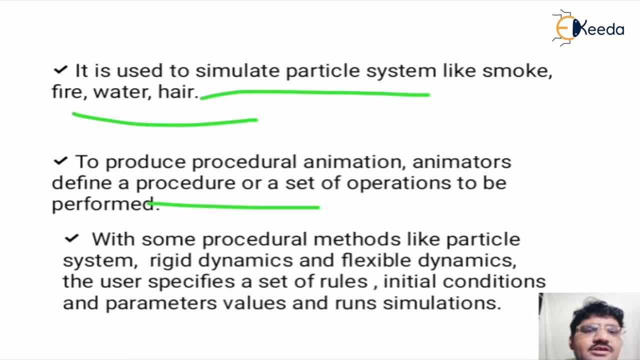 set of operations to be performed. That's why this animation is called procedural animation. With some procedural methods like particle systems, rigid dynamics and flexible dynamics, the user specify a set of rules, initial conditions and the parameters values- and run simulations. So now discuss all these. 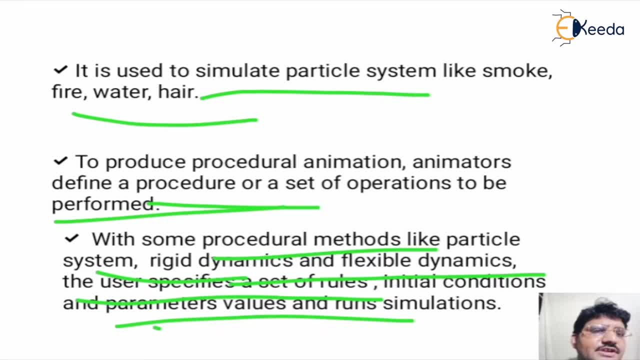 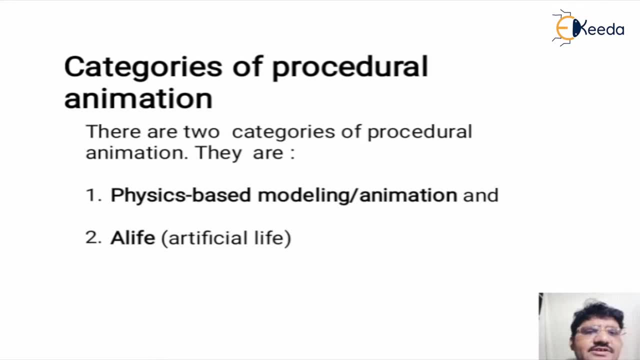 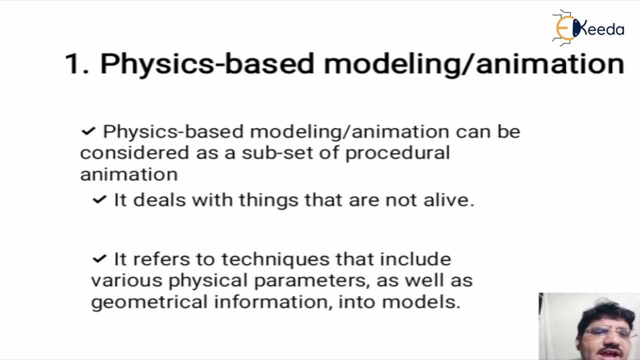 procedures in detail. The procedures can be classified in two categories. First one is physics based modeling- animation- and the second is LI, for artificial life. Physics based animation, modeling or animation can be considered as a subset of procedural animation. This method deals with things that are not alive. 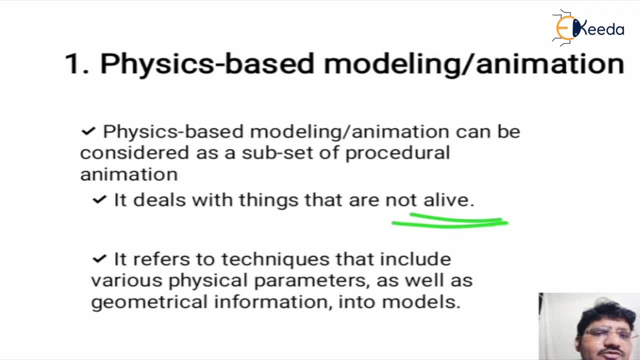 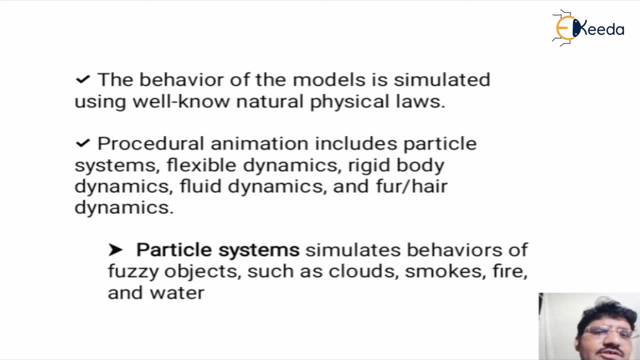 It refers to techniques that include various physical parameters as well as geometrical information into models. The behavior of this model is simulated using well known natural physics law. Procedural animations include particle systems, flexible dynamics, rigid body dynamics, fluid dynamics and hair dynamics. 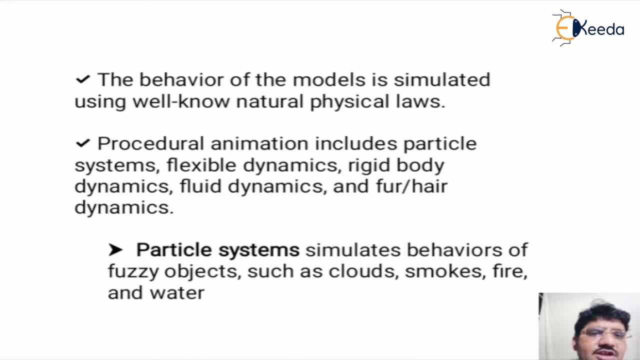 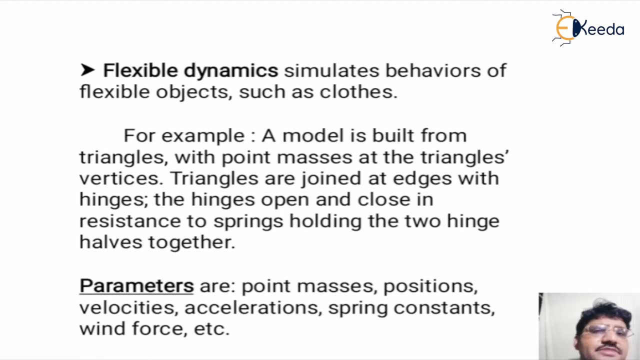 Let's see what are these. Practical systems simulate behavior of fuzzy objects such as cloud, smoke, fire and water. Flexible dynamics simulate behavior of flexible objects like cloths, For example. a model is built from triangle which points masses at the triangle. 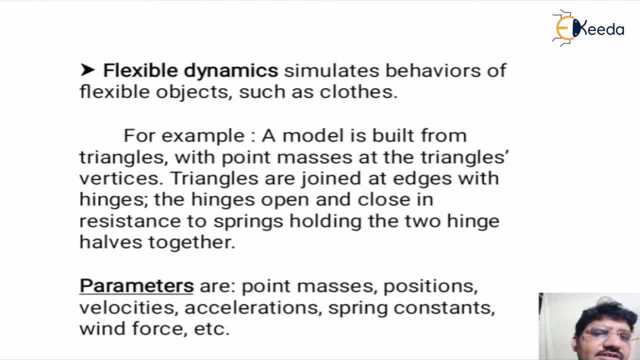 Triangles are joined at edges with hinges. The hinges open and close in resistance to spring, holding the two hinges held together. For this method the parameters are point masses, positions, velocities, accelerations, spring, constant wind force, etc. In the rigid body. 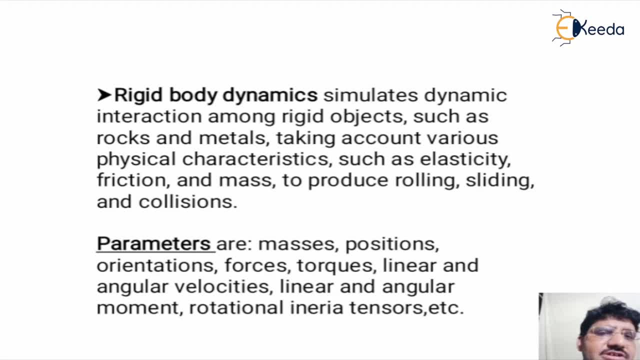 dynamic. we simulate dynamic interaction among the rigid objects like rocks and metals, Taking account various physical characteristics such as elasticity, friction, mass, to produce the rolling, sliding and collision effect. In this method, the parameters are masses, position, orientation, forces, torque, linear and angular velocities. 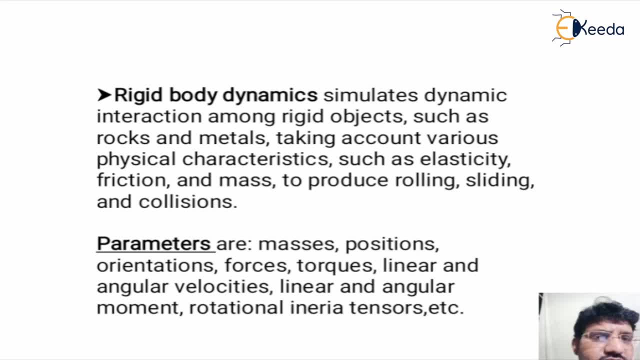 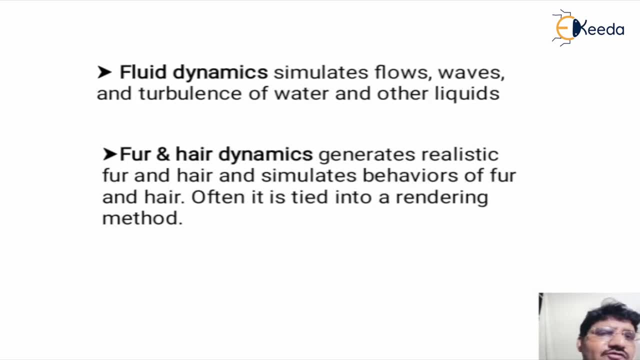 linear and angular movement, rotational tensor, etc. In the fluid dynamic we simulate flow wave and turbulence of water and other liquids. In the hair dynamics we generate realistic fur and hair and simulate behavior of fur and hair. It is tied into. 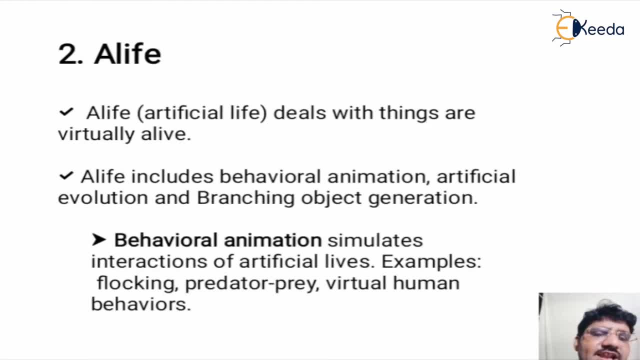 a rendering method. In the second, alive or artificial life it is deal with things are virtual alive In this method. things are in virtual In the previous method. the things are in physical Alive includes behavior, animation, artificial evolution and branching object generation.